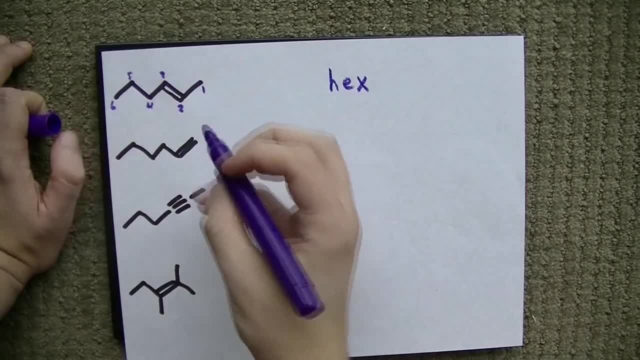 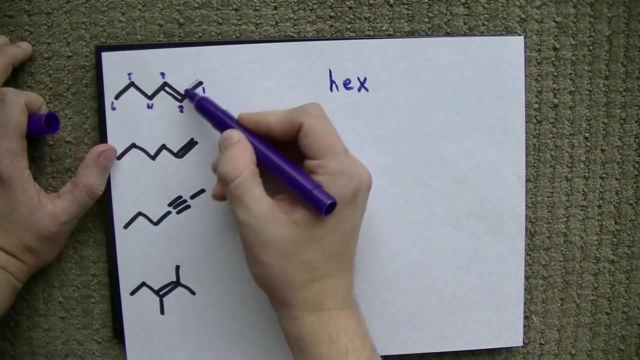 labeled it from zero, we would have a double bond. So if we labeled it from the other direction, it'd be one, two, three, four and two is the lower number, So we prefer two. Now, this double bond could have been between the first two carbons. it could have been between the third and the fourth carbon, but no, it's. 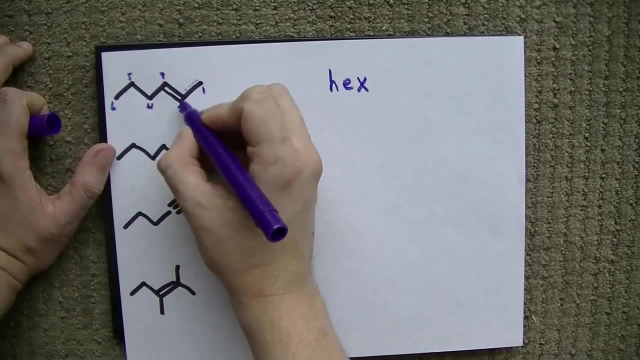 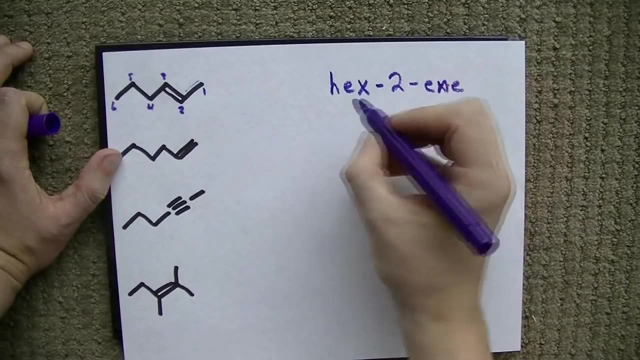 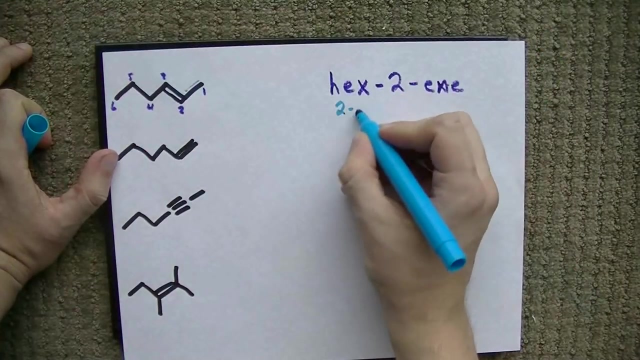 here. We have to tell people that the double bond starts at carbon two, And so we call this hex, two ene. That's H-E-X, dash two, dash E-N-E. Now some teachers who are using an outdated naming system might call it two hexene. But the IUPAC, the group of 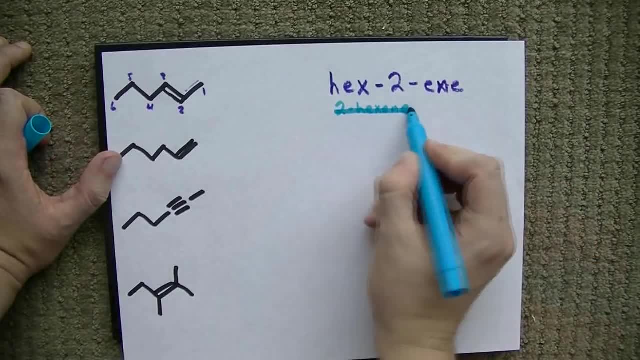 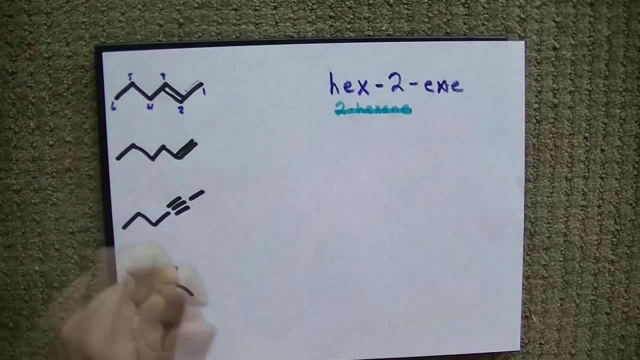 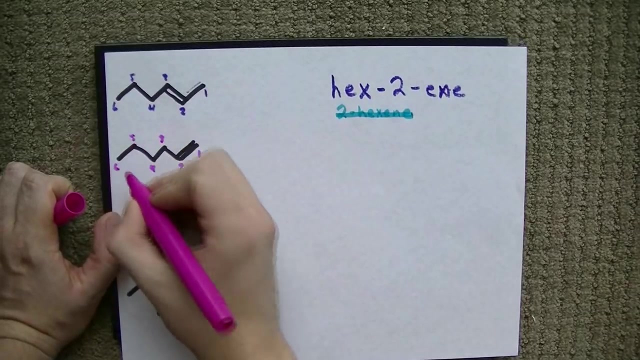 Swedish people who control how we name things. we don't use that anymore. We put the two in front of the ene to show that's where the double bond is. Let's try this again. We've got one, two, three, four, five, six carbons in a chain, So again it's a hex. And the double 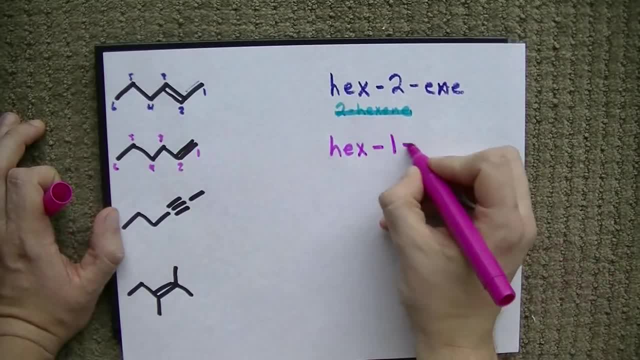 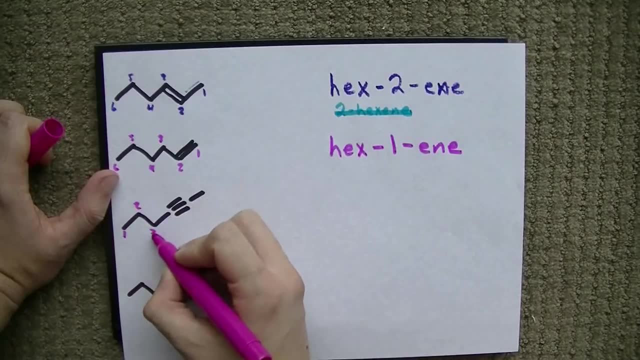 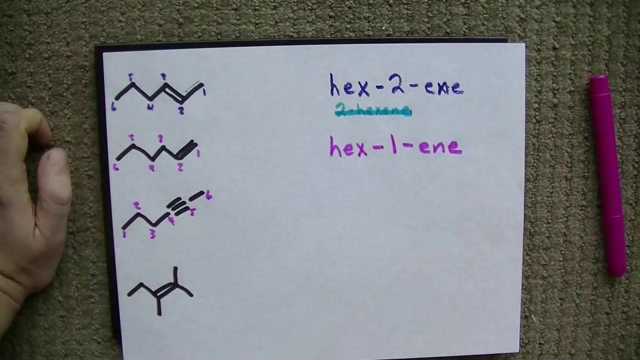 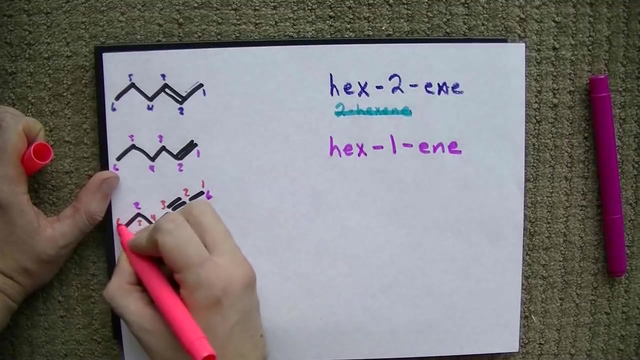 bond starts at carbon number one. So this is hex one ene. Pretty straightforward, eh. One, two, three, four, five, six. Oh no, I think I labeled this in the wrong direction. we could have labeled it one, two, three, four, five, six and the. 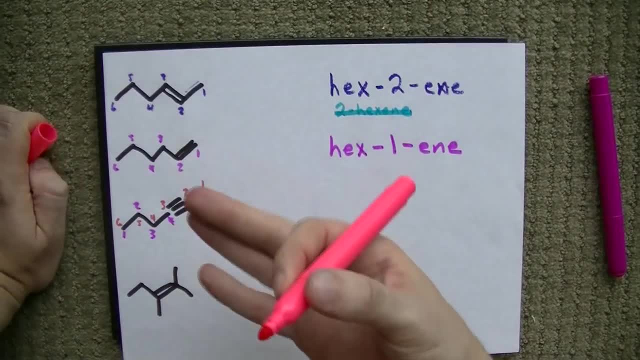 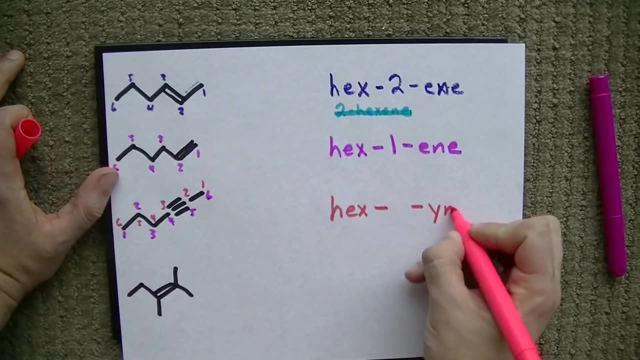 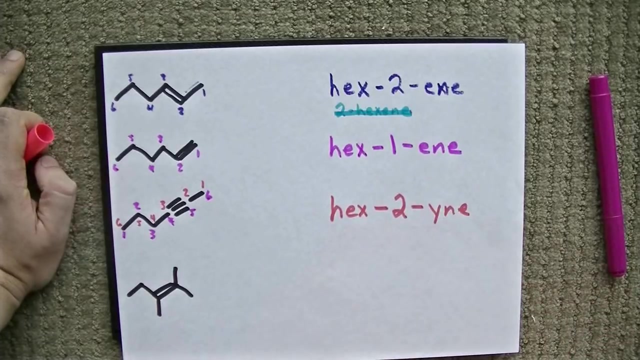 triple bond would have started at carbon two. Again, we prefer the lower, lower numbers. So six carbons, hex, and we have a triple bond starting at carbon number two, hex 2-ine. Pretty cool, Let's do this last one. It's a little branched. What color do I want to? 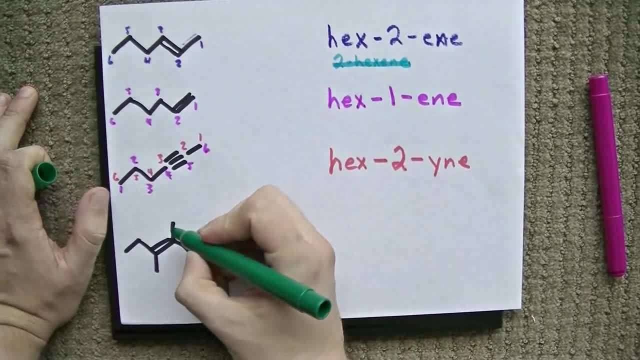 use What's the longest carbon chain here: 1, 2,, 3,, 4, 5,. 1, 2, 3, 4, 1, 2,, 3,, 4, 5.. Looks like. 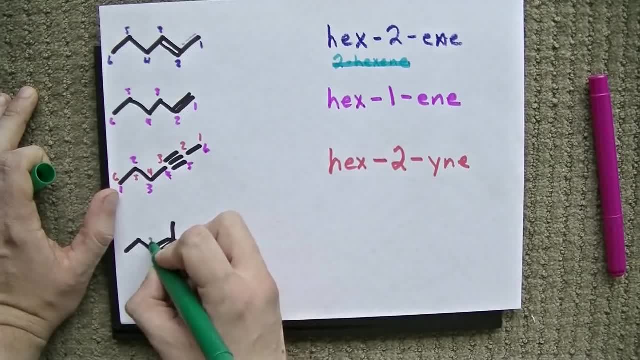 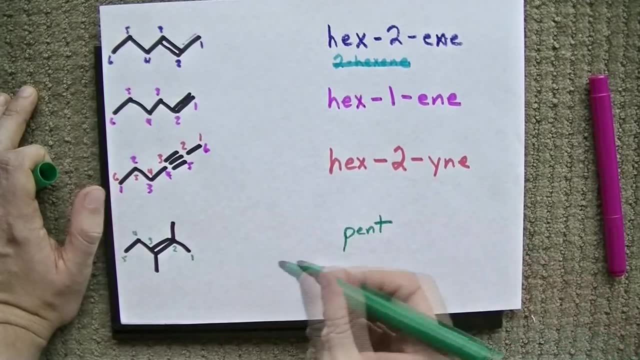 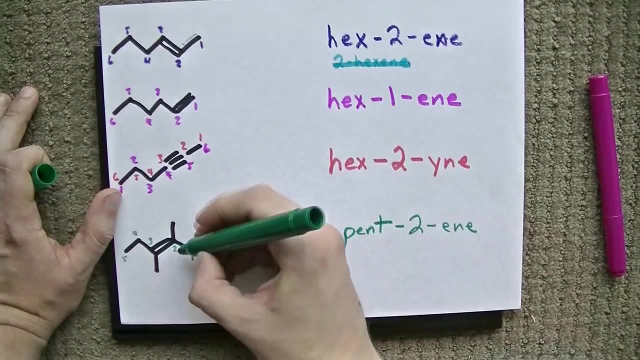 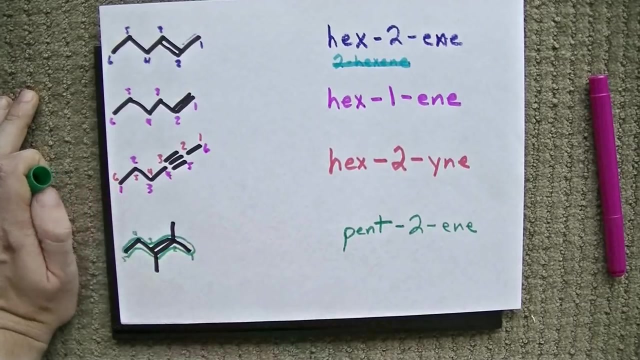 it's just five: 1,, 2,, 3,, 4, 5.. That makes this a pent-ine. The double bond, or ine, starts at carbon 2, so it's pent-2-ine and that takes care of these carbons in the chain in the five carbon. 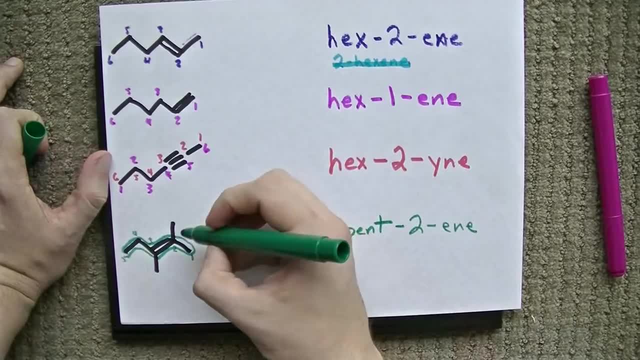 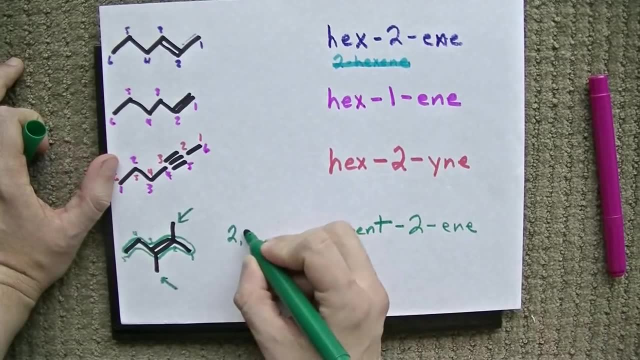 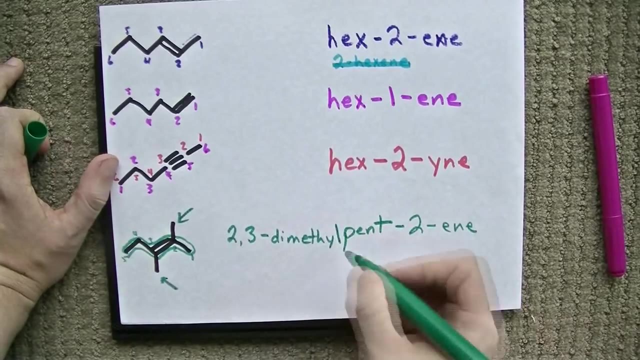 chain. Now we also, you might notice, have single carbons, Two carbon chains hanging off of carbons two and three in the chain. That's why we need to add a 2, 3 dimethyl. There's no space in between methyl and pentene, So we have a five carbon chain with 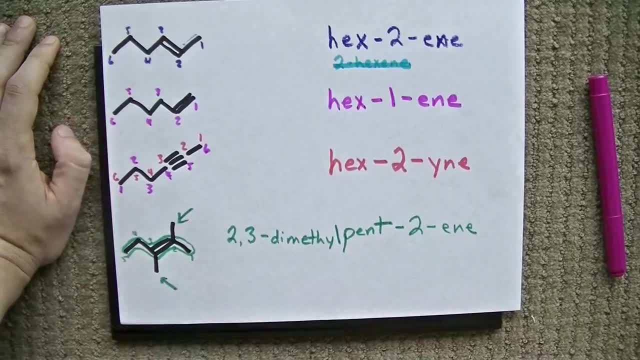 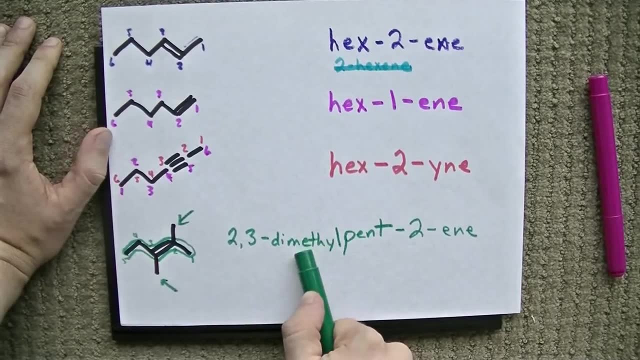 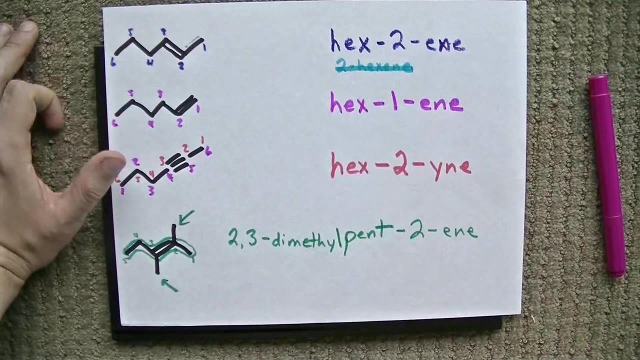 a double bond. starting at carbon number two, Check, And also off of carbons number two and three, we have single carbon chains, or CH3 groups. Two, three, dimethyl pent-2-ine. Pretty cool, Good job naming that with me, guys. Now for you, advanced folks. 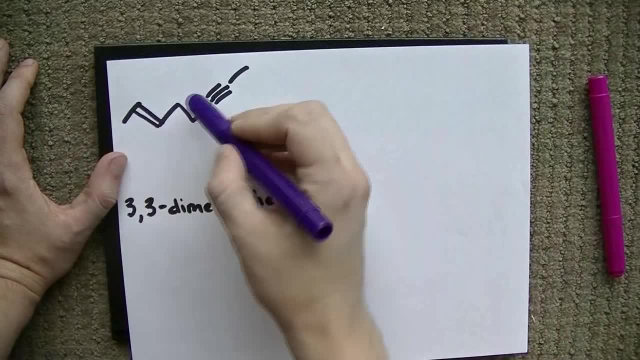 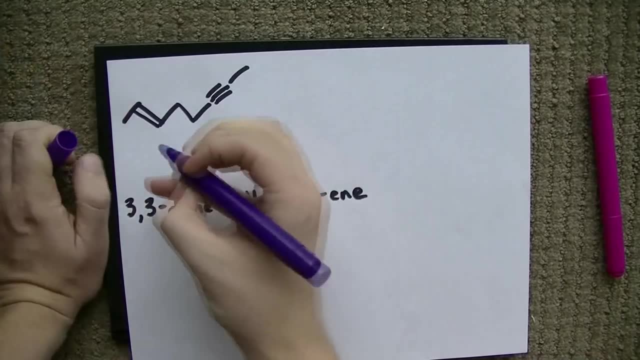 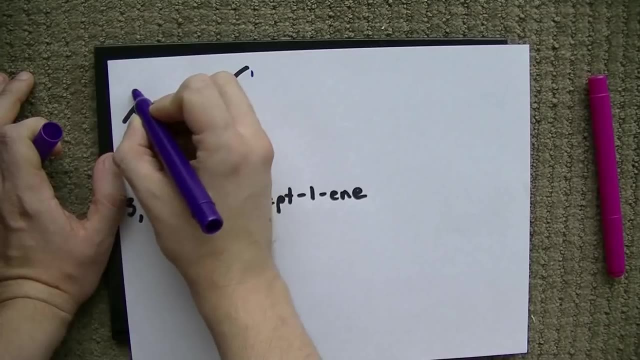 you may see a molecule that has a double bond and a triple bond. What we do is we include both suffixes. Here's what I mean. We've got carbon 1, 2, 3, 4, 5, 6, 7, 8.. This is definitely an oct. 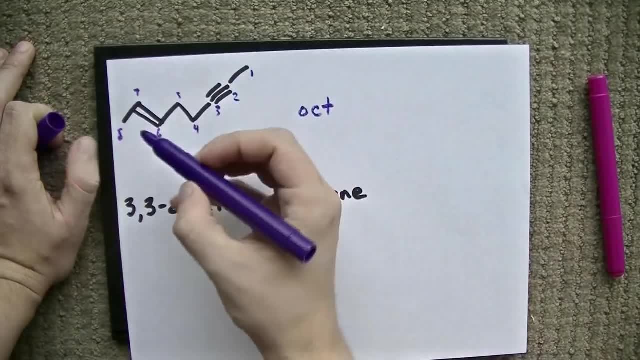 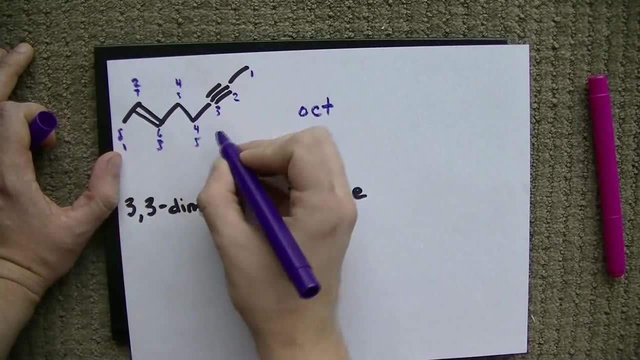 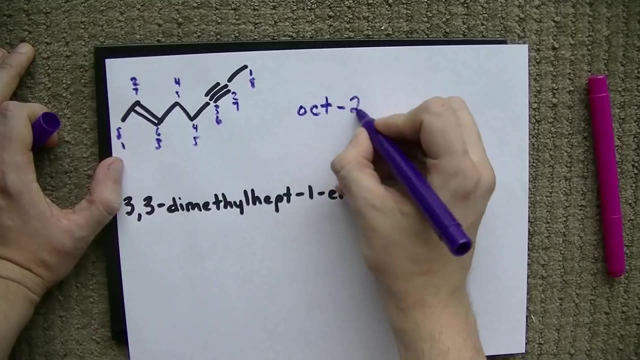 But we have a double bond, starting at carbon. Uh-oh. 1,, 2, 3.. See how I always have to figure out which one has the lowest number. I'm gonna give the in the lowest number here: Oct. 2-ine and 6-amine. 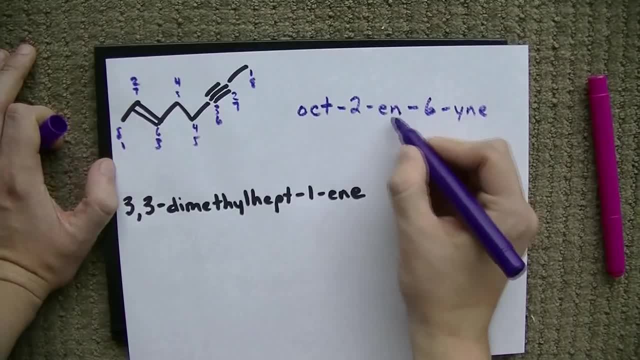 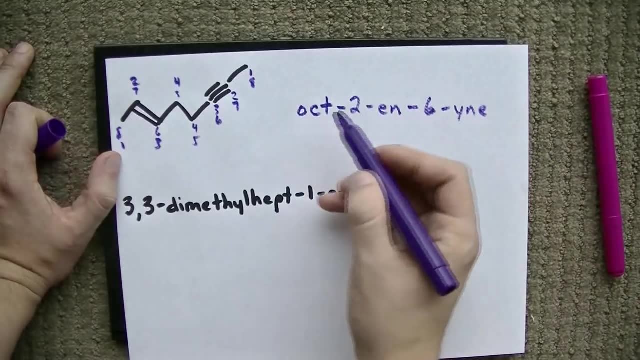 Now there's this thing where if you have anything after the in, you're supposed to cut off the extra E just trust me on that for now. and we have oct 2-ene 6-yne. This shows us we have an 8-carbon chain with a double bond and a triple bond. The 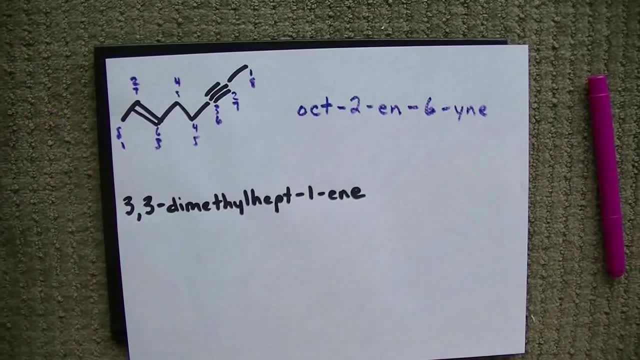 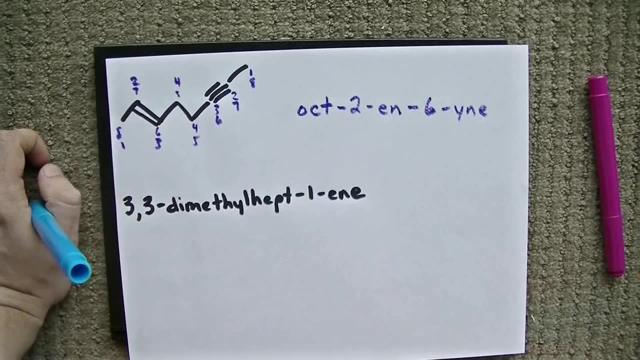 double bond starts at carbon 2,. the triple bond starts at carbon 6.. Now for those of you who are even more advanced than that, you may be asked to tell people whether the molecule is cis or trans. I'm going to make a separate video. 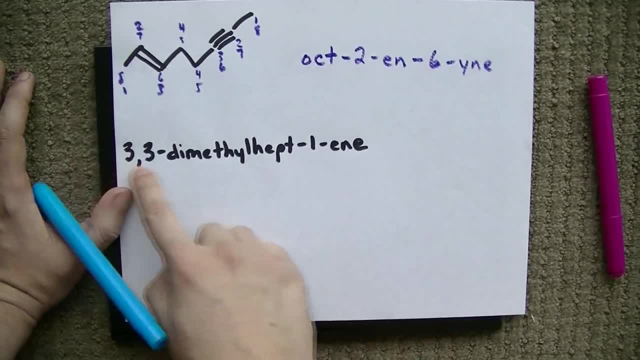 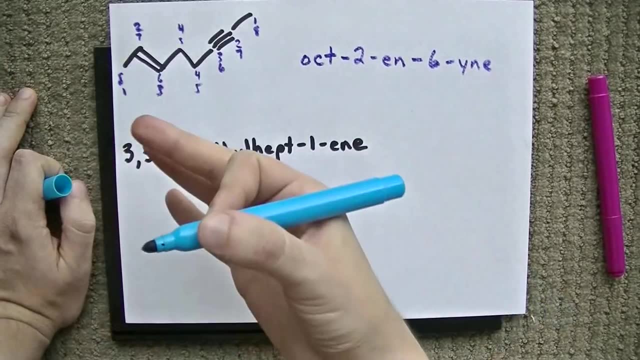 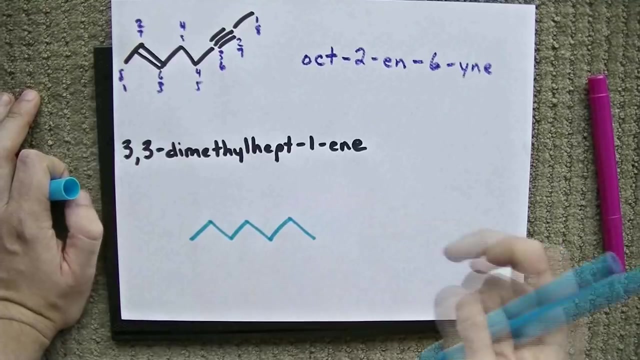 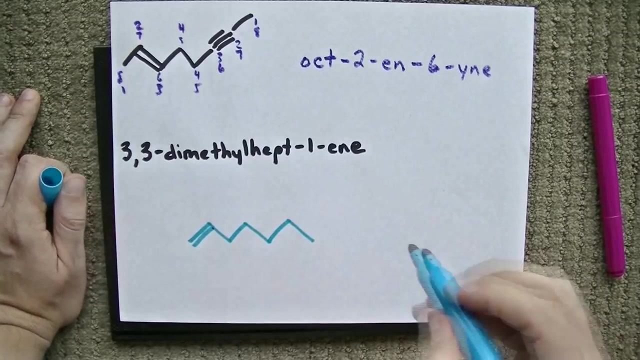 for that. For now, I need you to draw this. Let me show you how I draw organic molecules. Hept means seven carbons in a chain: One, two, three, four, five, six, seven, Starting at carbon 1, I have a double bond, Carbon 1,, double bond, And I have. 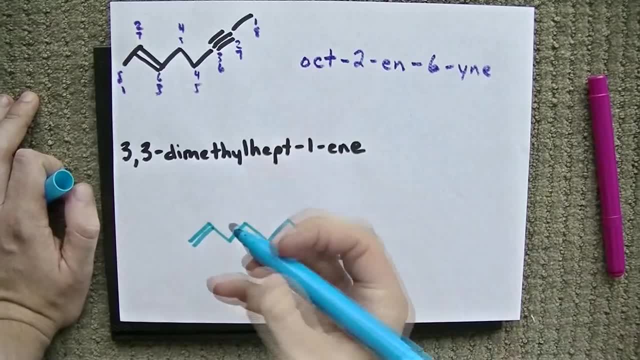 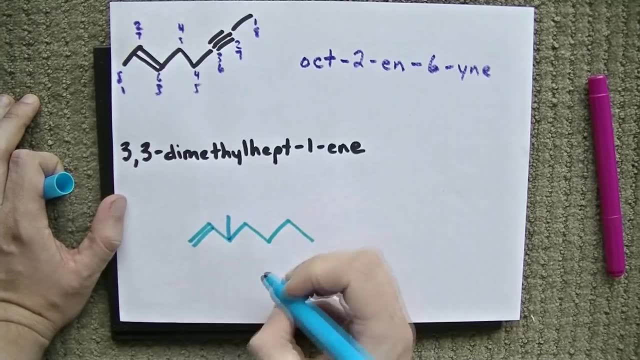 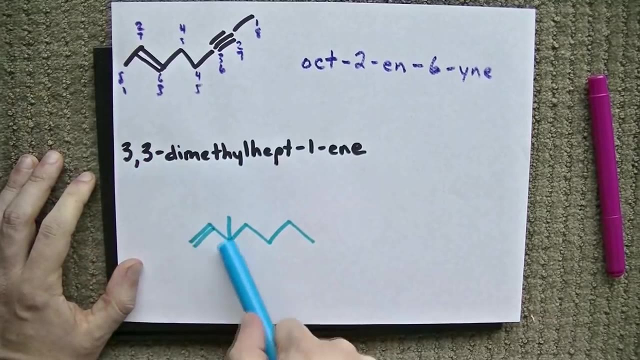 two methyl groups, that's, single carbon chains hanging off of carbon- 3, and three. We called this carbon 1,, 2, and 3 before, so I'm going to put a CH3 here and a CH3 there: 3, 3-dimethyl-hept-1-ene. It's a beautiful thing. The last thing I 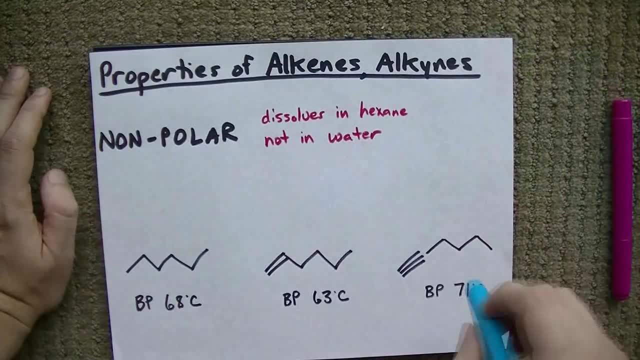 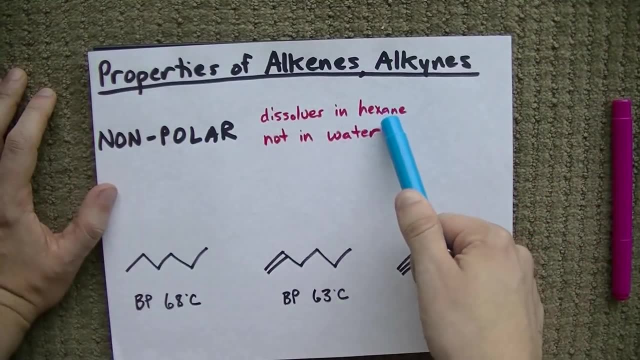 want to point out are some of the properties of alkenes and alkynes. It's still only carbon and hydrogen, so it's generally nonpolar, which means it'll dissolve in nonpolar solvents like hexane, but not in. 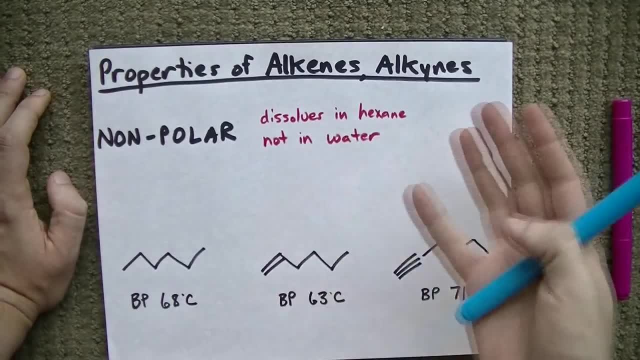 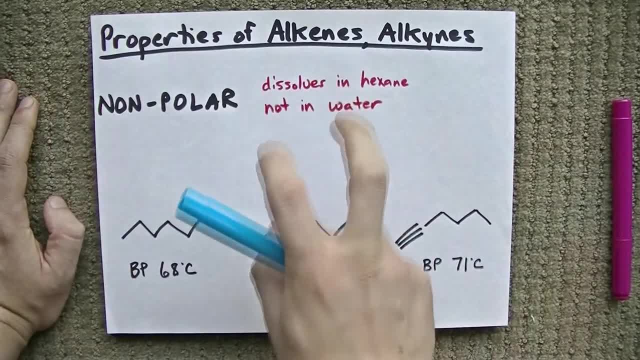 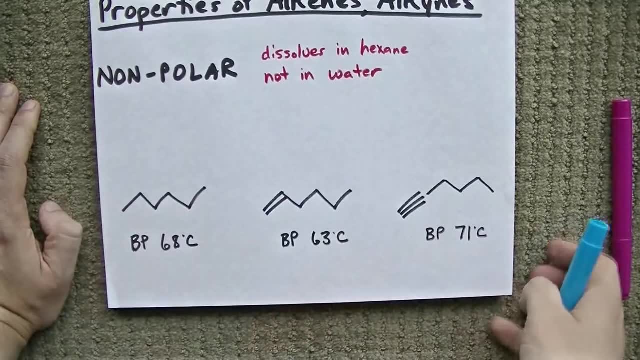 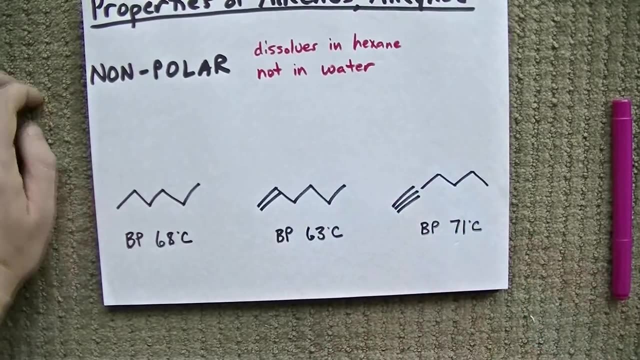 they're basically pretty much the same: Alkene, alkene, alkene, alkene, alkyne, Like. take a look at the boiling points of hexane: one hexene and one hexyne. They're all pretty comparable, but this is a trend for all of them, The alkenes. 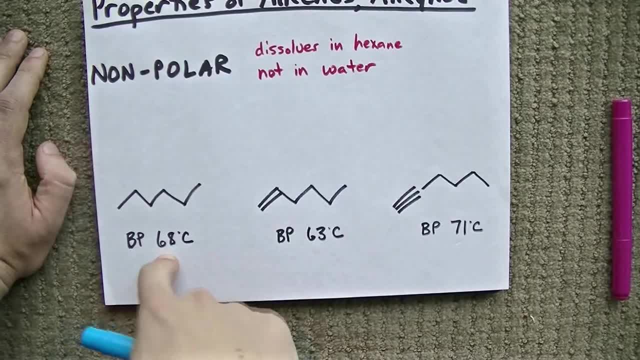 have slightly lower bonds than the alkenes. The alkynes have slightly higher boiling points than the alkenes. The alkynes have slightly higher boiling points than the alkenes. Let me reword that The highest boiling point among the three goes to the alkyne. 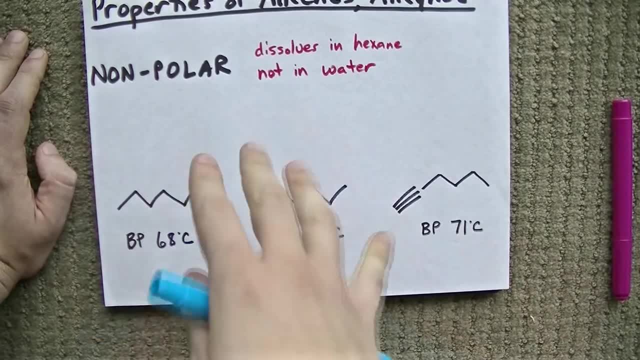 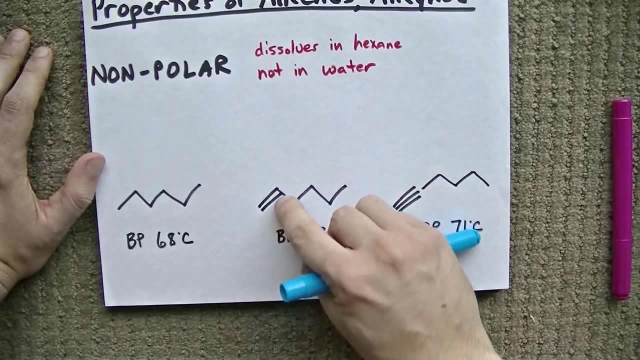 and the lowest one goes to the alkene. The alkene is somewhere in between. Now, I don't exactly know why this is the case. I think it has to do with the fact that, the way this bond is, it doesn't allow the molecules to be packed as closely together. 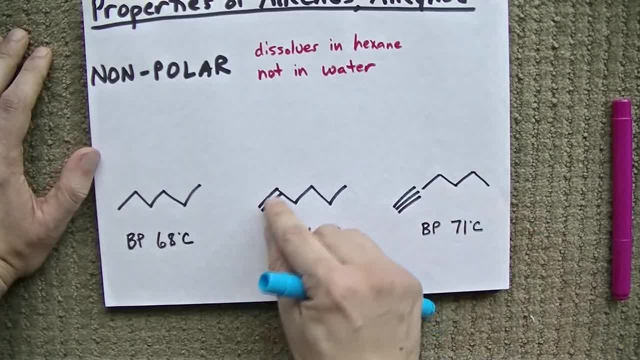 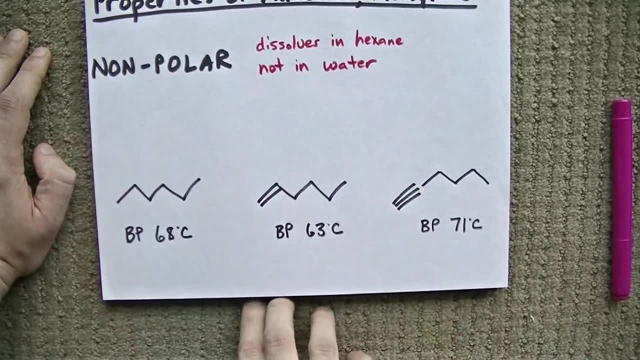 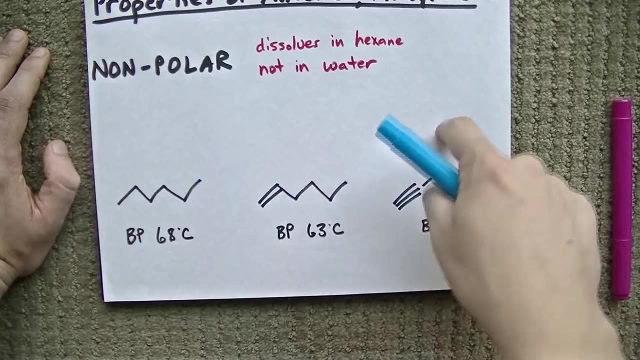 as this or this, just because of the arrangement of the atoms around the double bond versus the triple bond or single bond. But don't quote me on that being the reason. Long story short, this has the weakest intermolecular forces: the alkene, and the alkyne is the strongest intermolecular forces.